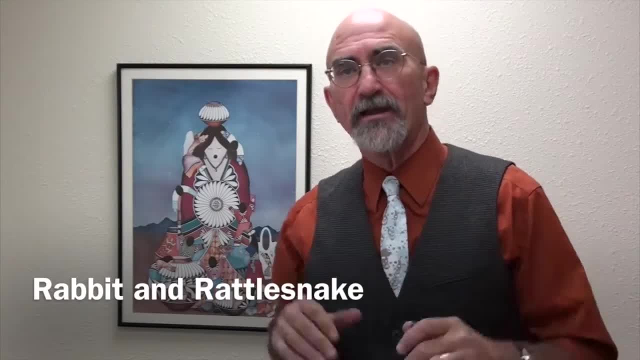 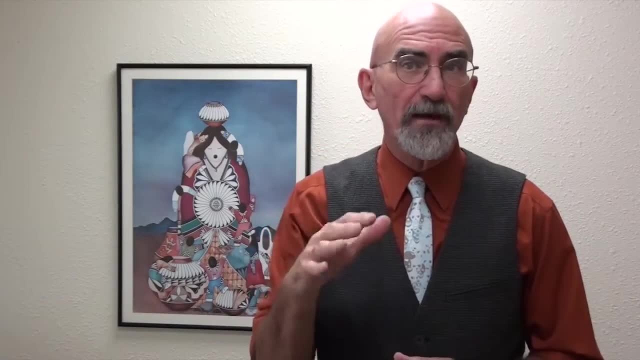 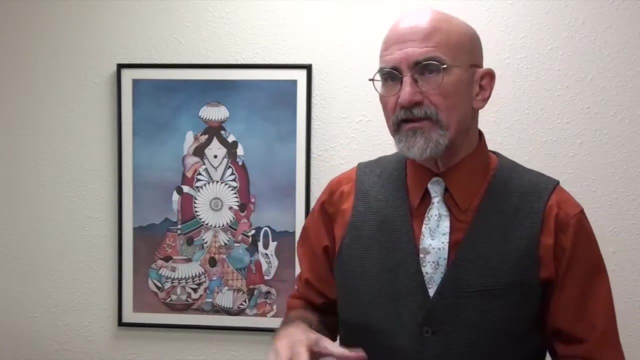 One morning Rattlesnake was lying on a ledge sunning himself after the cold night warming up, and he opened up an eye and he saw coming in the distance rabbit. and he thought to himself this could be good for me. and so he looked around real quick and he saw over on that side of that ledge. 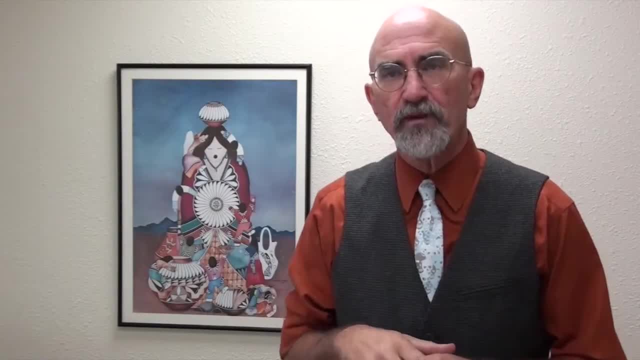 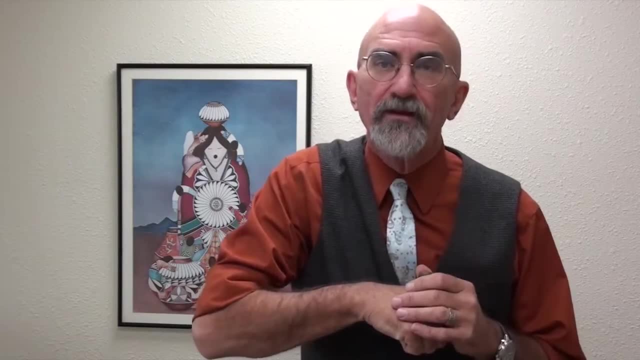 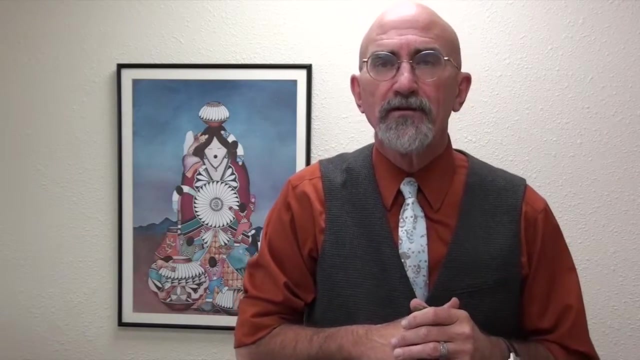 there was a stone that sort of stuck out from the mountain and had just a little bit of a gap underneath it. so he slithered on over there and pushed himself into that gap and he called out: rabbit, rabbit. rabbit looked up and said: what do you want? rattlesnake said: i need some help, i'm stuck. 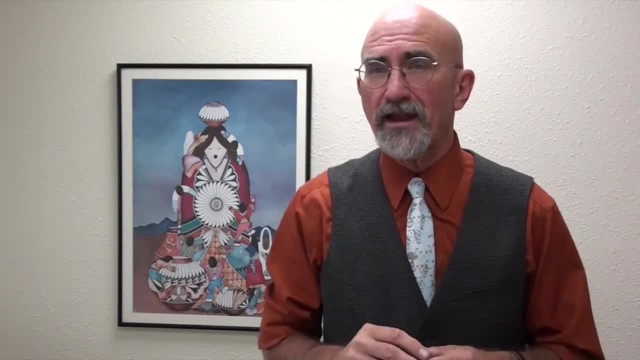 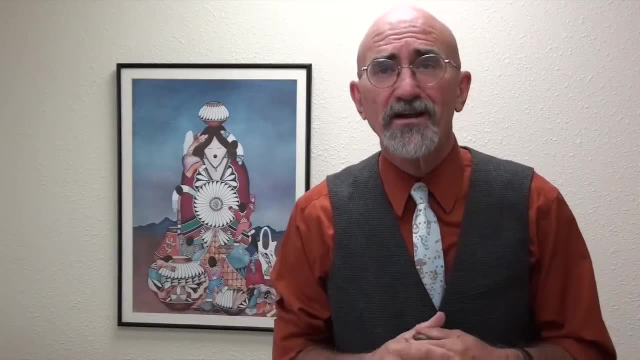 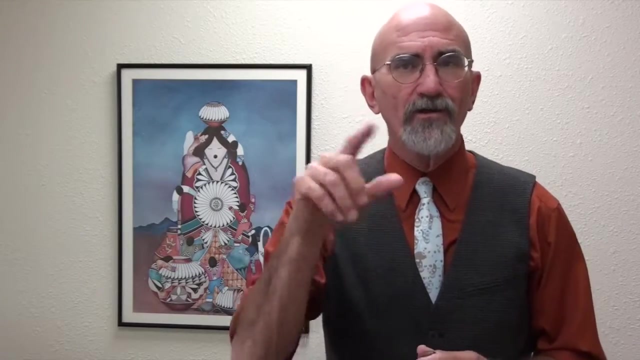 and rabbit says: you're not going to get that help from me. and rattlesnake says: oh yeah, i need your help. you're the only one that's come by in a long time. this rock fell on me and i'm stuck. can you please lift up the rock and get me out? and rabbit said: i don't think so. i know very well that. 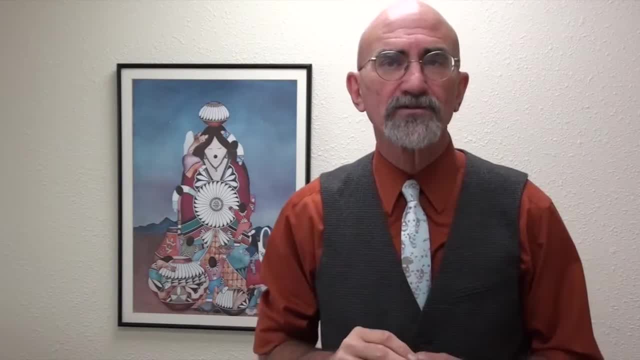 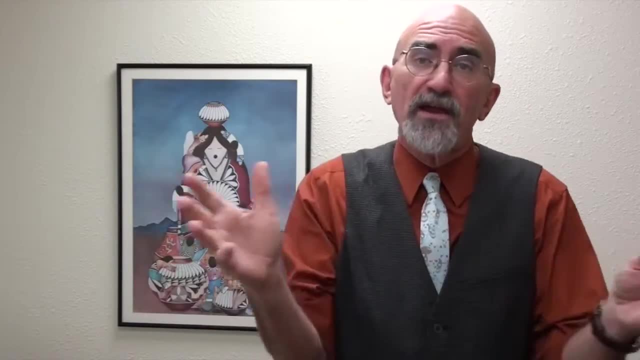 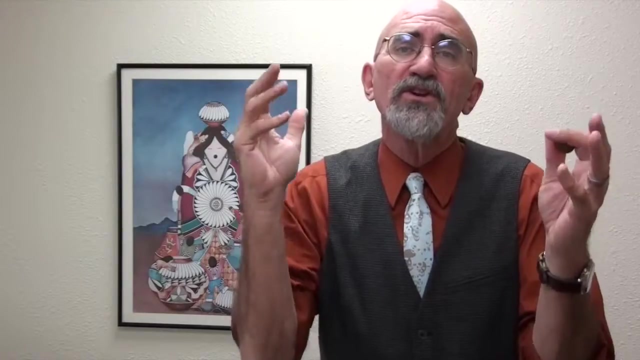 rattlesnakes eat rabbit and i don't feel like coming close enough. and rattlesnake said: eat rabbits, not now a normal situation. i might be thinking that way, but look, i'm stuck, i need help. and in order to have help, i promise you i would never hurt you, like that rabbit said. why should i believe your promises? 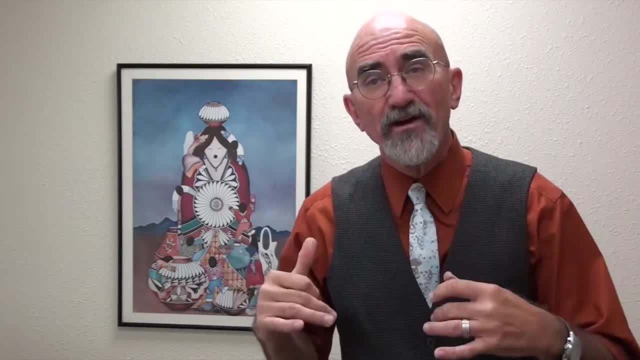 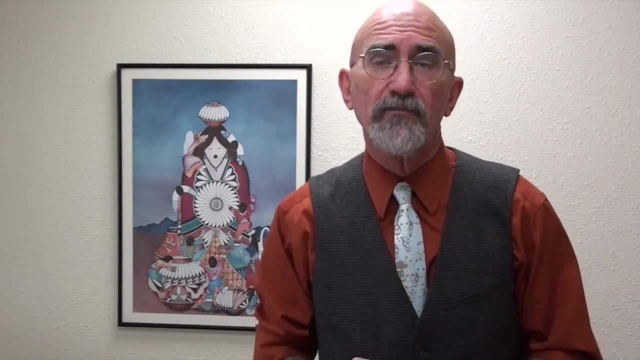 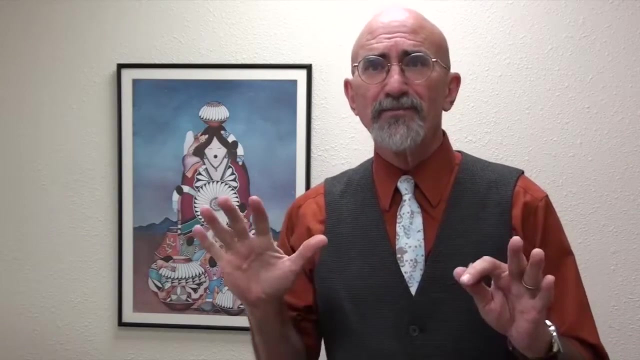 and rattlesnake said: because when a person needs help, they need a friend, and when a friend, when someone becomes a friend, you don't treat friends badly by lying to them. please help me lift this up. rabbit says you promise you won't try anything. rattlesnake says i promise you'll be my friend. so rabbit hopped up on the ledge and he went over and 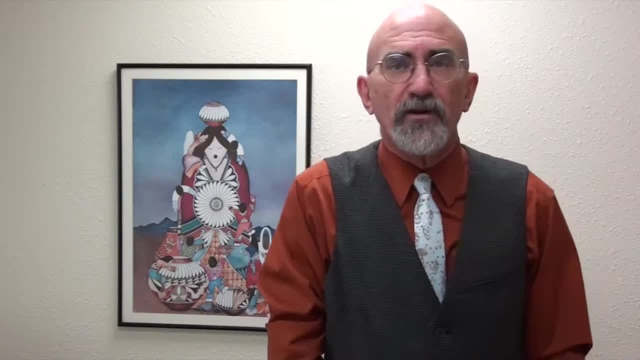 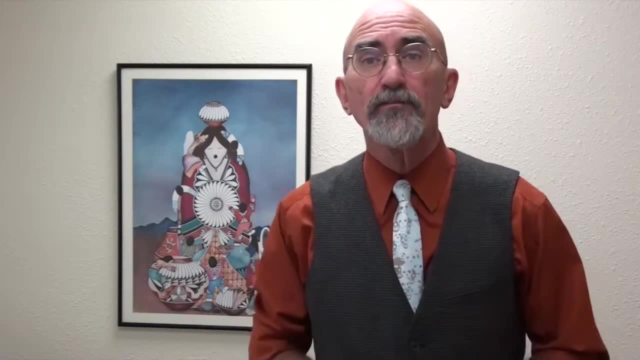 he tried lifting up their rock and rattlesnake slid out from underneath and said: that was just enough, thank you so very much. and rabbit turned back around and rattlesnake said: now prepare to be my lunch. and rabbit said: wait a minute. you promised me you wouldn't do that. and he said: 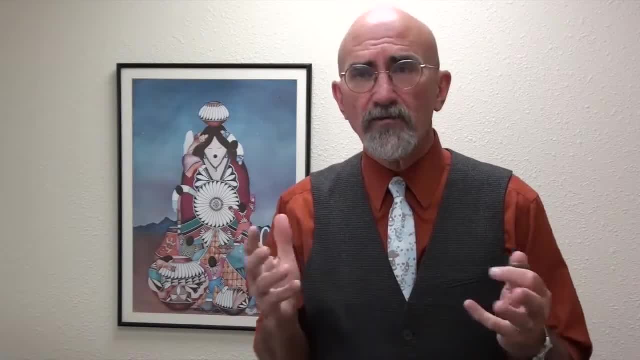 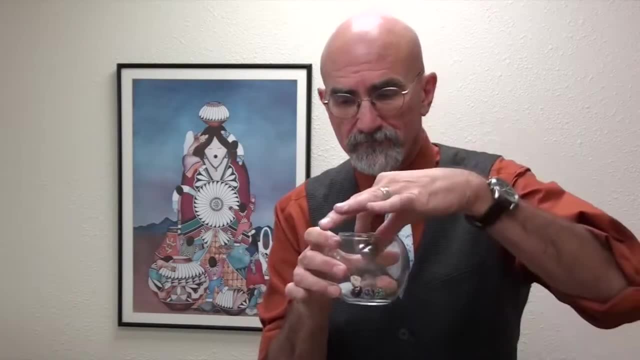 don't do anything like that. and rattlesnake said: but i'm a rattlesnake, that's what rattlesnakes do, and that is my story.